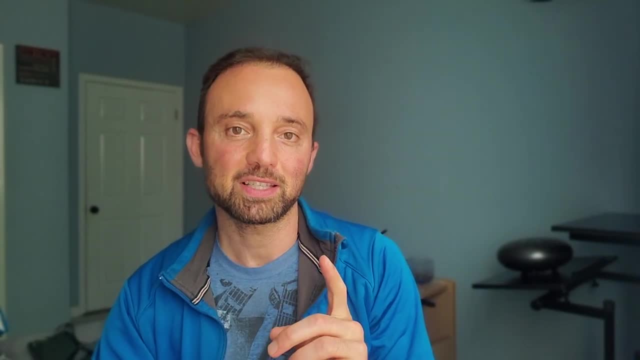 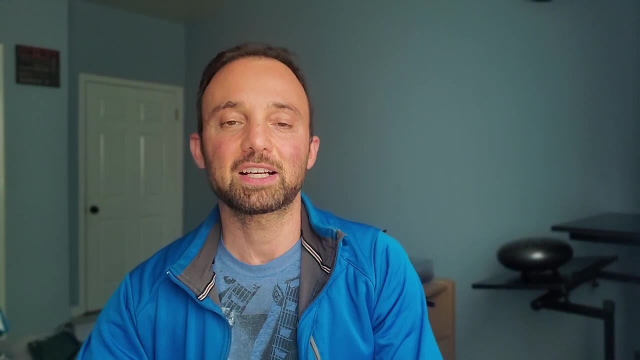 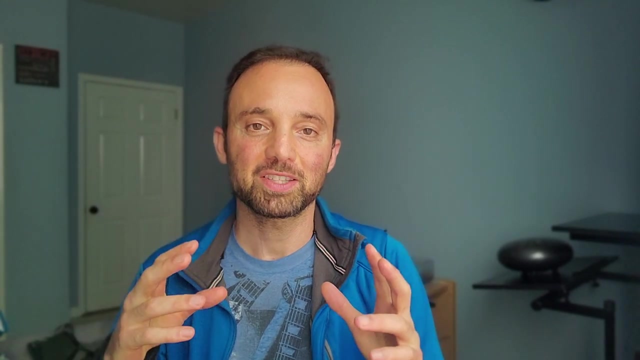 you can make, and i've done one video about this in the past that i'll link in the description to in this video, and i am going to do another video coming up where i show even more lifestyle factors and fundamental changes that you can make to increase your hrv. now, before i get to the 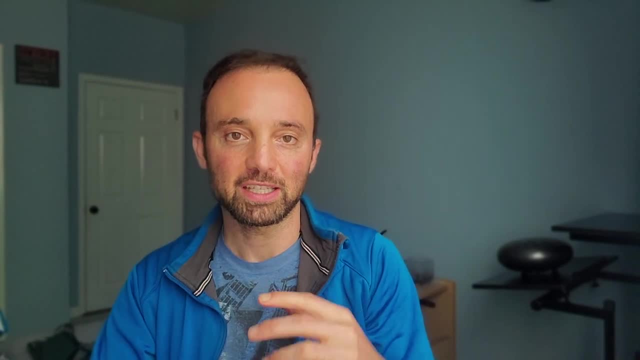 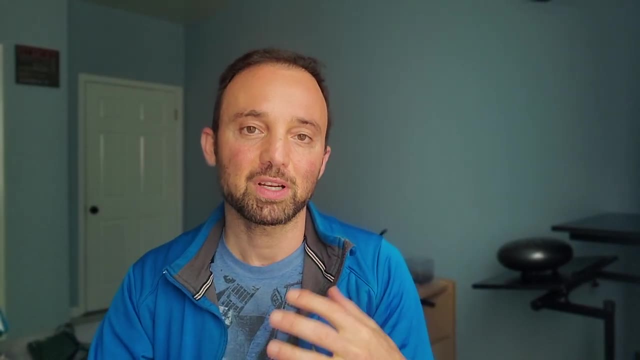 numbers that you can compare your current hrv against some of the ranges that were done in a study and let you know whether you're in the optimal or normal range. i want to talk about a study that was done some time ago that you may have seen out there on the internet. 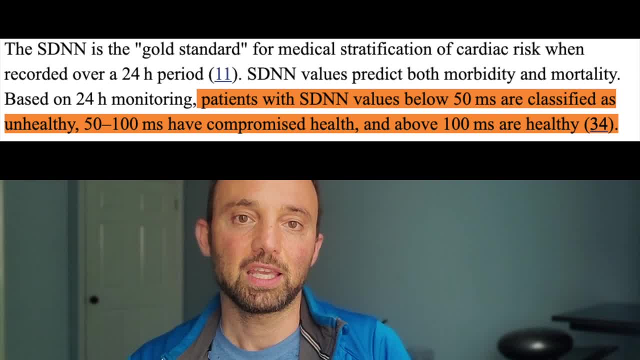 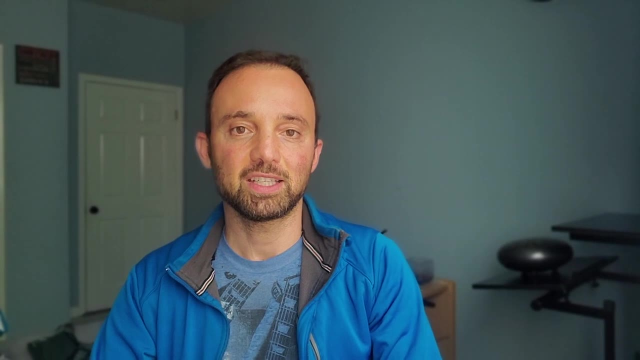 now, what this study says is that if your hrv is between 0 and 50, you are in poor health, if your hrv is between 50 to 100, you have compromised health, and if your hrv is above 100, then you are in good health. now, what i do want to mention about this study is that a it uses sdnn. 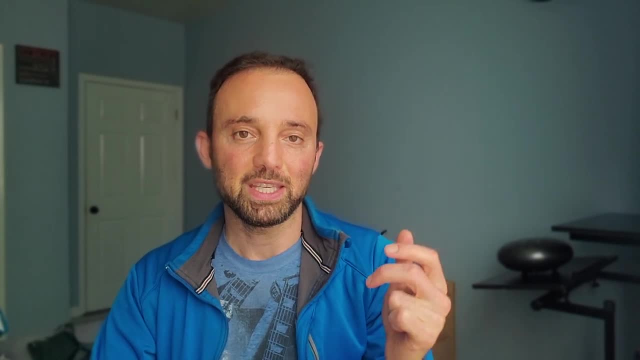 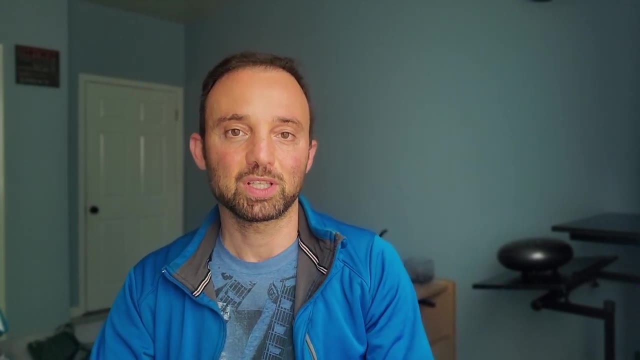 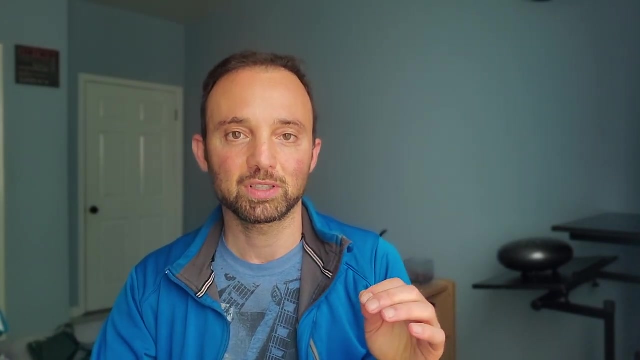 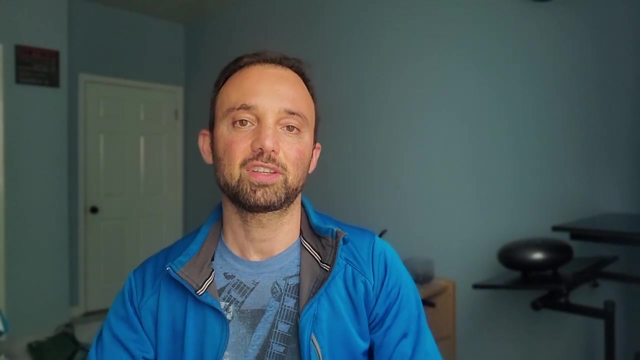 which we talked about a little bit earlier in the video and b. this was done over a 24 hour time period and apple watch does not do readings over 24 hour consistently. and lastly, this study was done on heart patients and it's particularly important for cardiovascular health, but hrv can actually be used for a broad range of health. so for now, 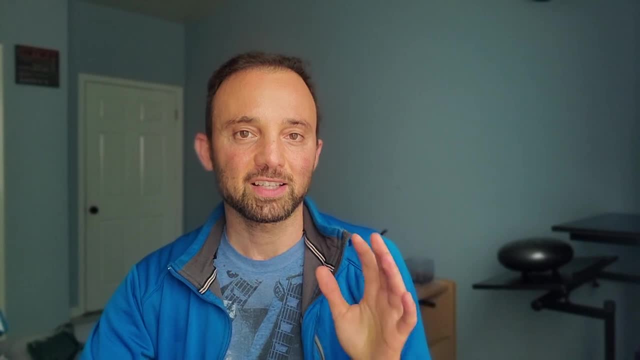 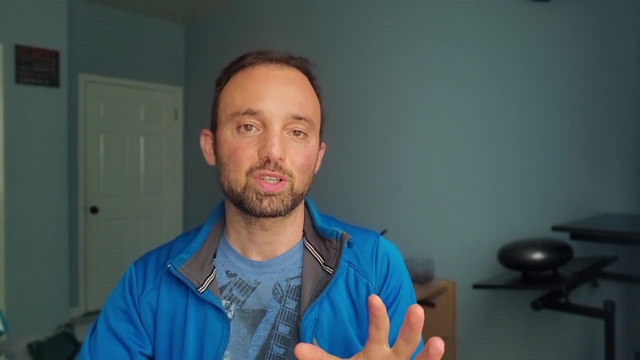 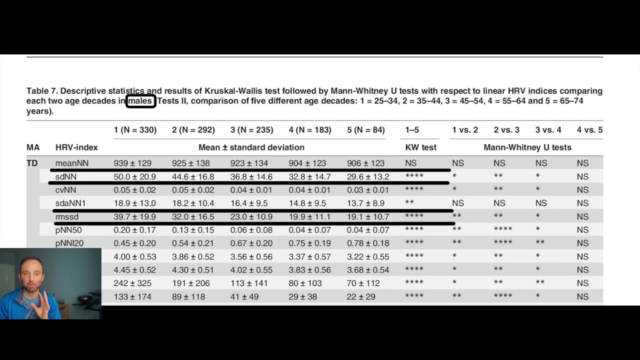 i wouldn't really worry about the results of this study unless you fit all the criteria that i just mentioned. i would like you to focus on the study that i'm about to show you, which shows hrv ranges for healthy people within certain age categories. all right, and the moment we've been waiting for. 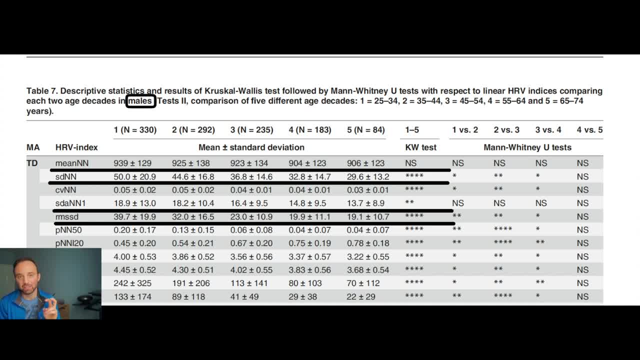 here the results of the study that show ideal numbers for hrv, and what we're going to do is we're going to find our age range and we're going to find the row that has rmssd for most wearables and that will be our ideal hrv range, and we're going to find the row that has rmssd for most.